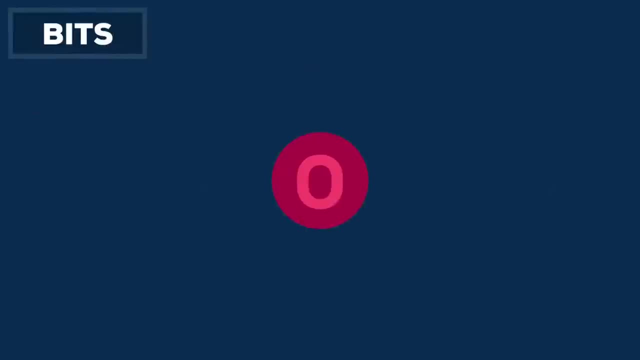 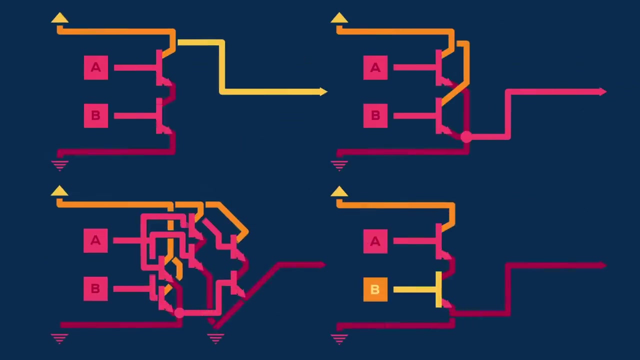 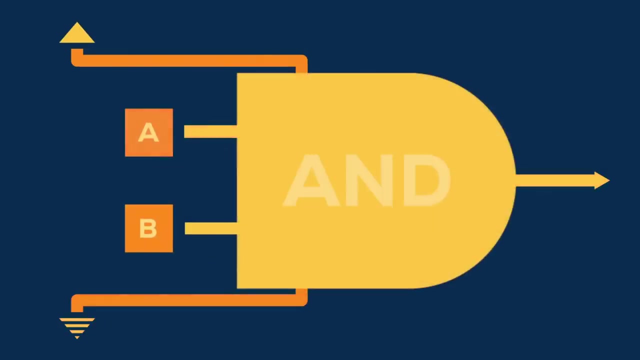 This information is made up of bits which can be set to either 0 or 1.. Combinations of several bits are used to represent more complex information. Transistors are combined to create logic gates which still do very simple stuff. For example, an AND gate sends an output of 1 if all of its inputs are 1,. 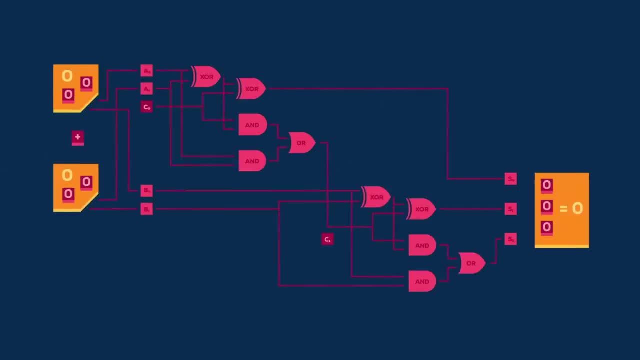 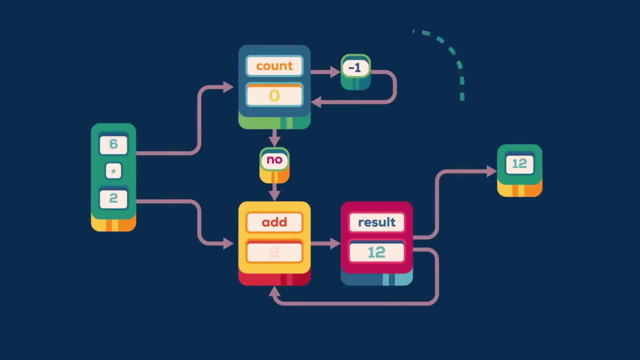 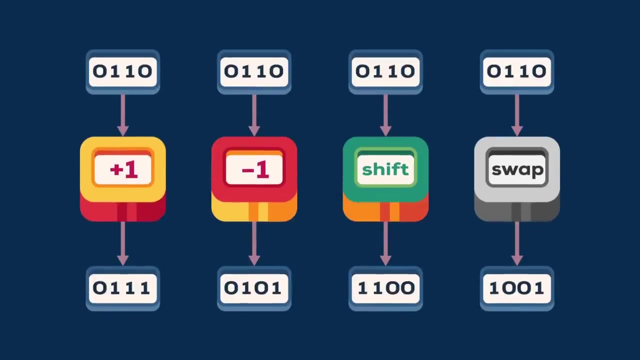 and an output of 0, otherwise Combinations of logic gates finally form meaningful modules, say for adding two numbers. Once you can add, you can also multiply, and once you can multiply you can basically do anything. Since all basic operations are literally simpler than first grade math, you can imagine a computer. 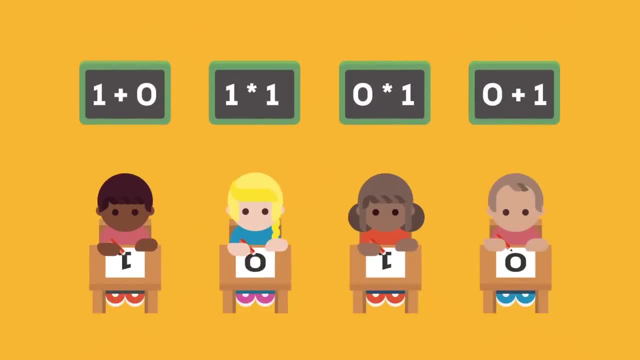 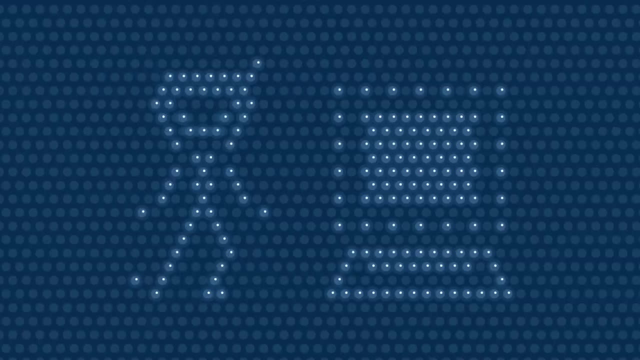 as a group of 7 year olds answering really basic math questions. A large enough bunch of them could compute anything from astrophysics to Zelda. However, with parts getting tinier and tinier, quantum physics are making things tricky. In a nutshell, a transistor is just a small tiny. 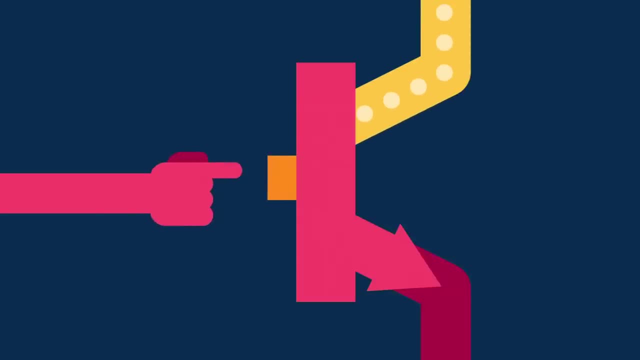 tiny transistor. Electricity is electrons moving from one place to another, so a switch is a passage that can block electrons from moving in one direction. Today, a typical scale for transistors is 14 nanometers, which is about 8 times less than. 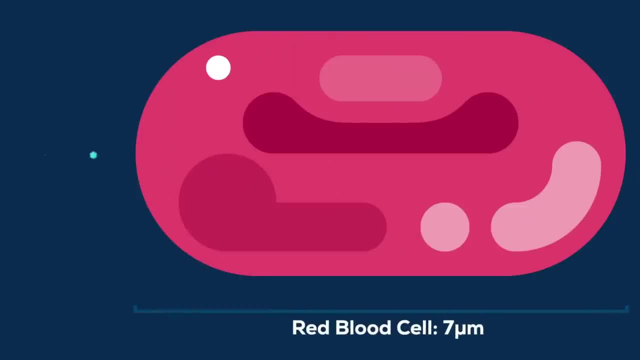 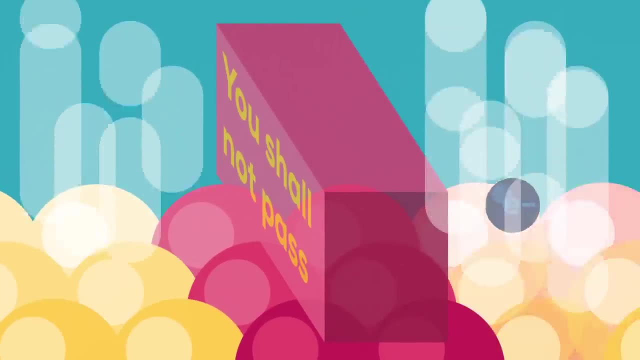 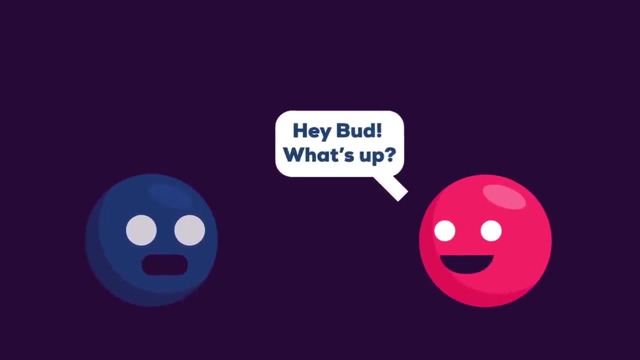 the HIV virus's diameter and 500 times smaller than a red blood cell's. As transistors are shrinking to the size of only a few atoms, electrons may just transfer themselves to the other side of a blocked passage via a process called quantum tunneling. In the quantum realm, physics works quite differently from the predictable ways. 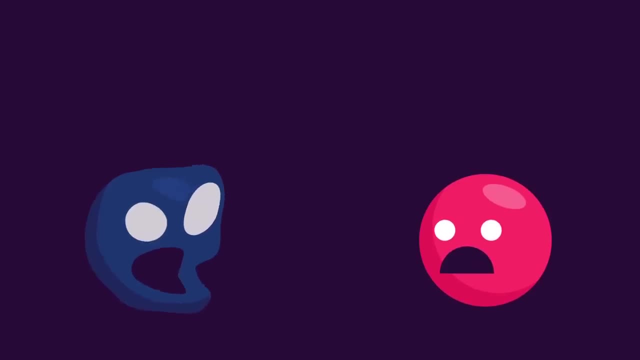 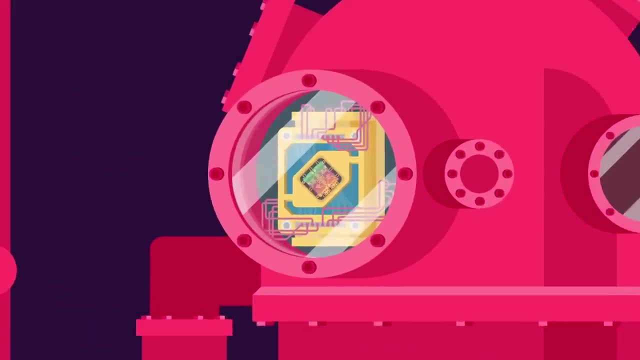 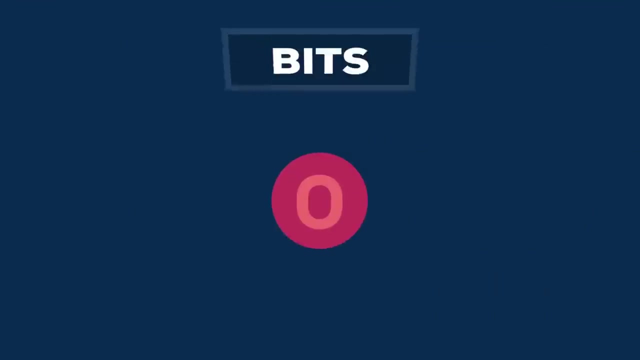 we're used to and traditional computers just stop making sense. We are approaching a real physical barrier for our technological progress. To solve this problem, scientists are trying to use these unusual quantum properties to their advantage by building quantum computers In normal computers. 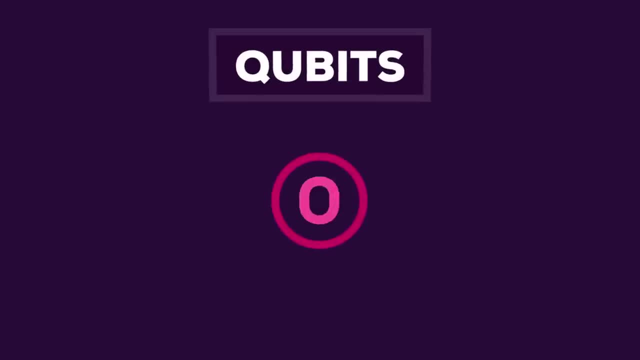 bits are the smallest units of information. Quantum computers use qubits which can also be set to one of two values. Quantum computers use qubits which can also be set to one of two values. A qubit can be any two-level quantum system, such as a spin in a magnetic field or a single photon. 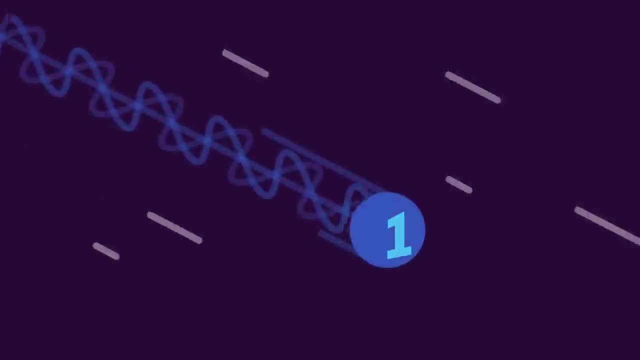 Zero and one are this system's possible states, like the photon's horizontal or vertical polarization In the quantum world. the qubit doesn't have to be in just one of those. it can be in any proportions of both states at once. This is called superposition. 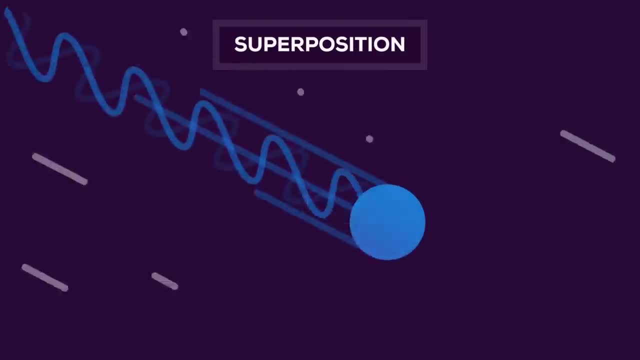 But as soon as you test its value, say by sending the photon through a filter, it has to decide to be either vertically or horizontally. So as long as it's unobserved, the qubit is in a superposition of probabilities for zero and one. 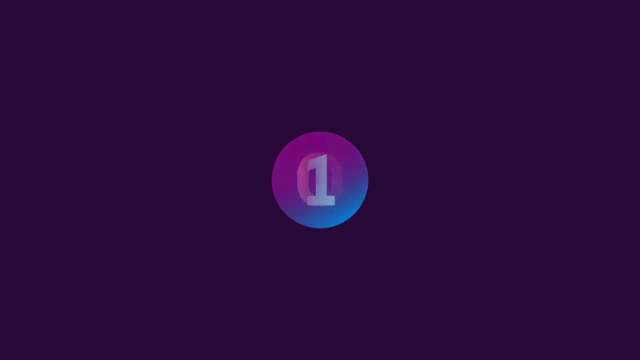 and you can't predict which it will be. But the instant you measure it, it collapses into one of the definite states. Superposition is a game-changer. Four classical bits can be in one of two to the power of four different configurations at a time. That's 16 possible combinations. 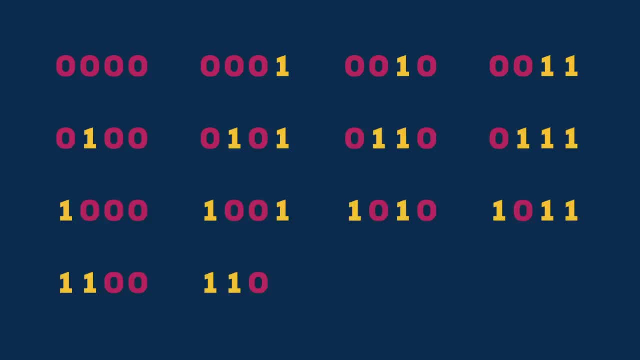 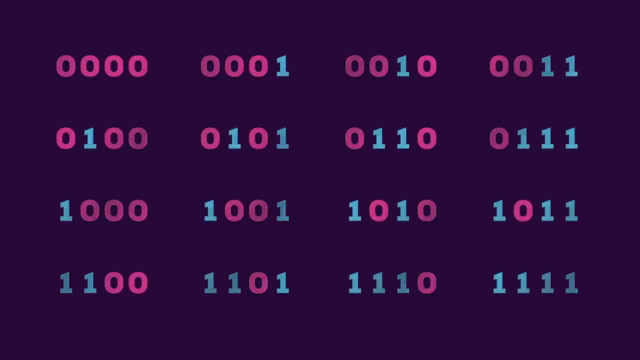 out of which you can use just one. Four qubits in superposition, however, can be in one of two or four different configurations at a time. That's quite a bit of a puzzle, all of those 16 combinations at once. This number grows exponentially with each extra. 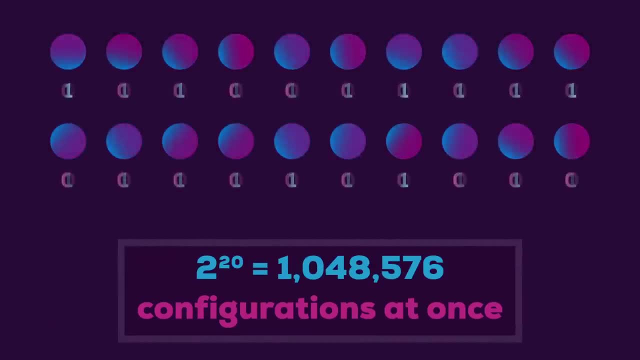 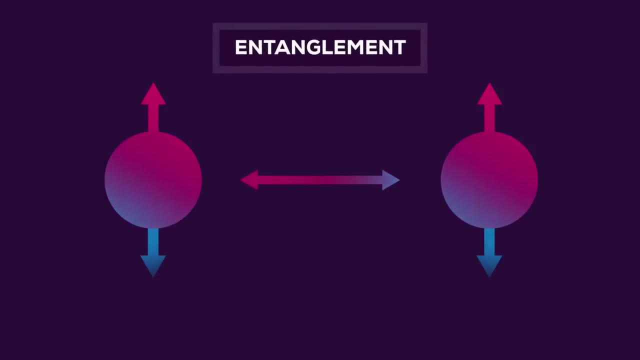 qubit. 20 of them can already store a million values in parallel. A really weird and unintuitive property qubits can have is entanglement, a close connection that makes each of the qubits react to a change in the other's state instantaneously. no, 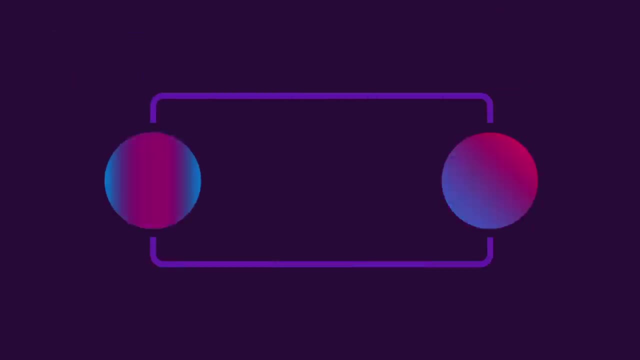 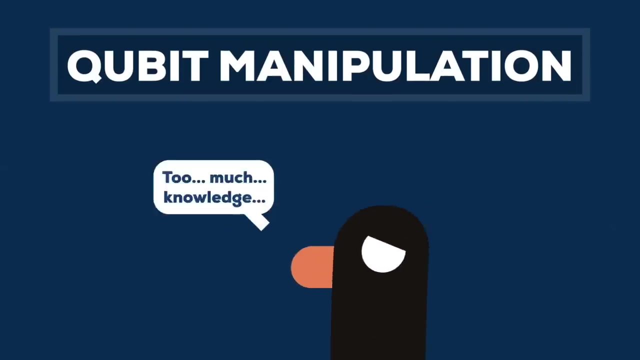 matter how far they are apart. This means that when measuring just one entangled qubit, you can directly deduce properties of its partners without having to look. Qubit manipulation is a mind-bender as well. A normal logic gate gets a simple set of inputs. 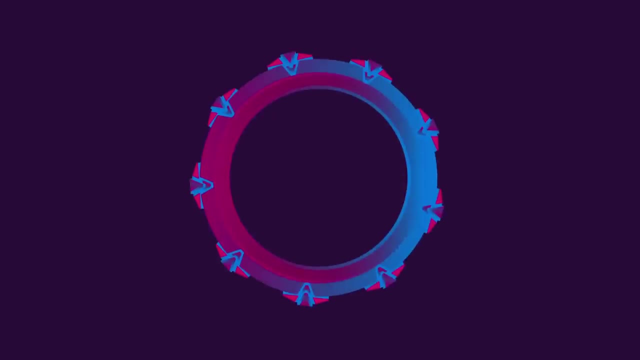 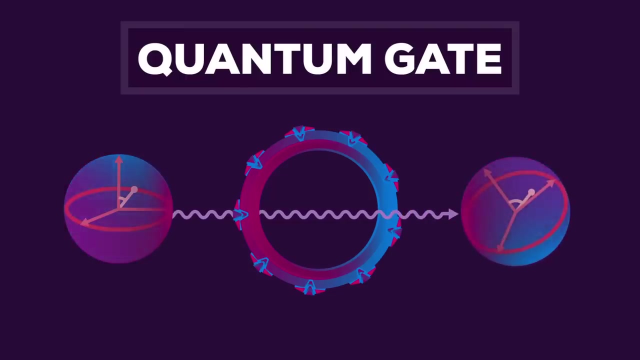 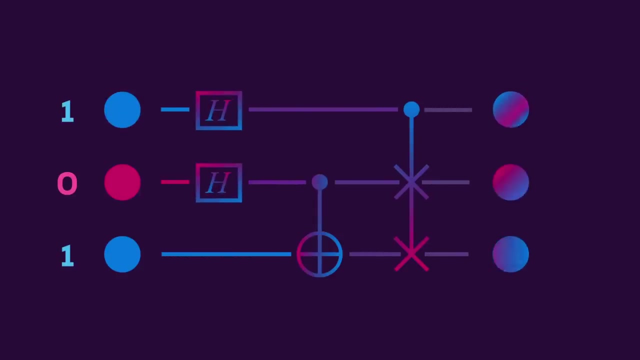 and produces one definite output. A quantum gate manipulates an input of superpositions, rotates probabilities and produces another superposition as its output. So a quantum computer sets up some qubits, applies quantum gates to entangle them and manipulate probabilities and finally measures the outcome. 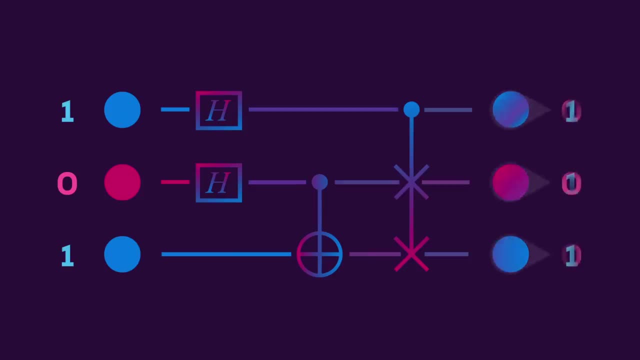 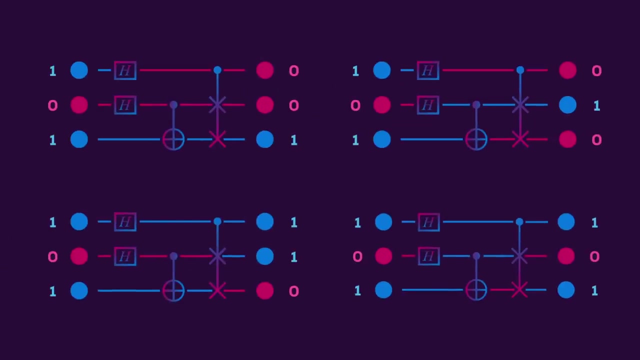 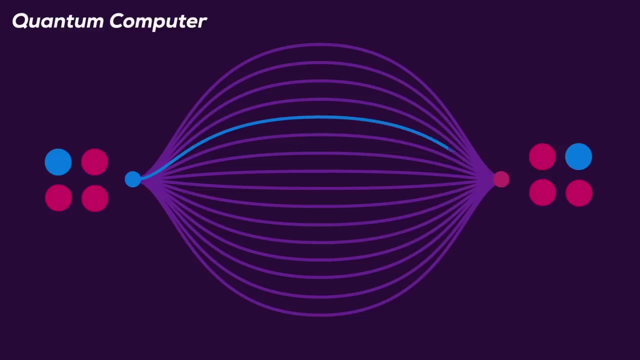 collapsing superpositions to an actual sequence of zeros and ones. What this means is that you get the entire lot of calculations that are possible with your setup all done at the same time. Ultimately, you can only measure one of the results and it will only probably be the one you want, so you may have to double-check and try again. 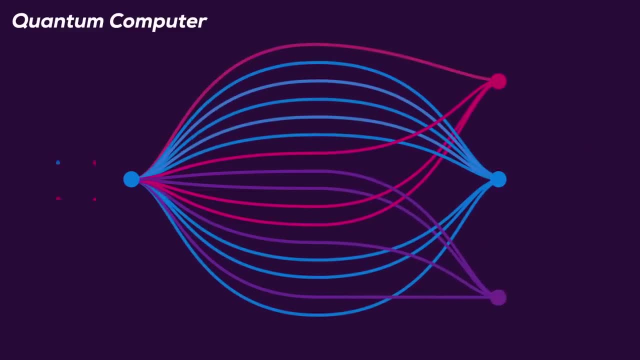 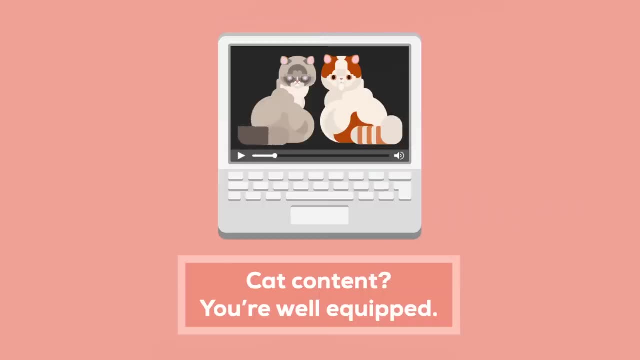 But by cleverly exploiting superposition and entanglement, this can be exponentially more efficient than would ever be possible on a normal computer. So while quantum computers will probably be able to do the same thing, quantum computers will probably be able to do the same thing on a normal computer. So while quantum computers will probably not replace our home computers, in some areas they are vastly superior. One of them is database searching. To find something in a database, a normal computer may have to test every single one of its entries. Quantum algorithms need only the square root.